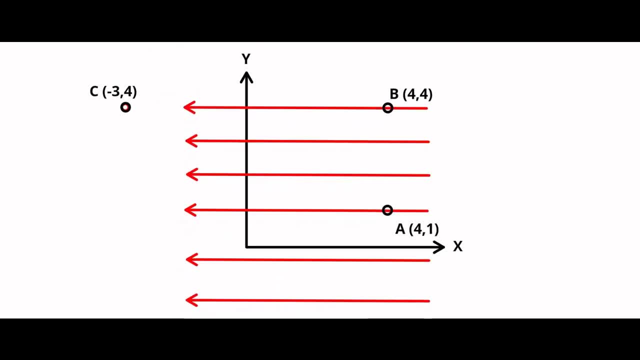 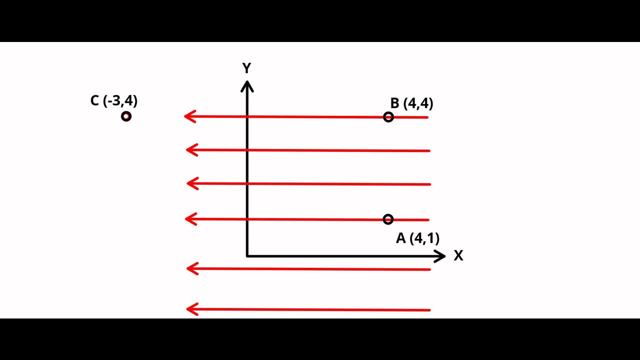 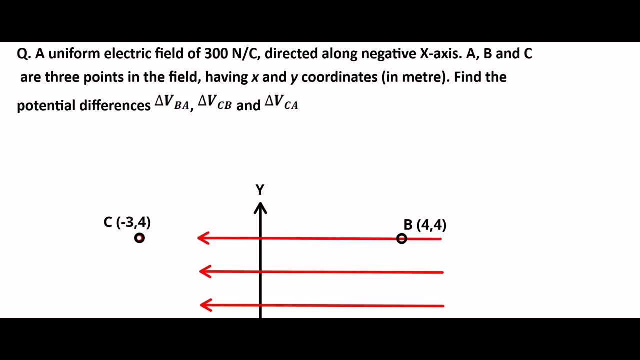 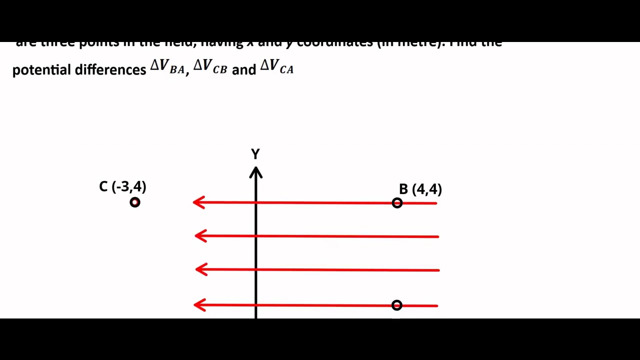 expressed as in this figure, This one electric field represented by the red arrows along the negative x-axis, and these are the three points A, B and C, And we have to find the potential difference between points B and A, that is, delta VBA, point C and B, delta VCB and point C and A. 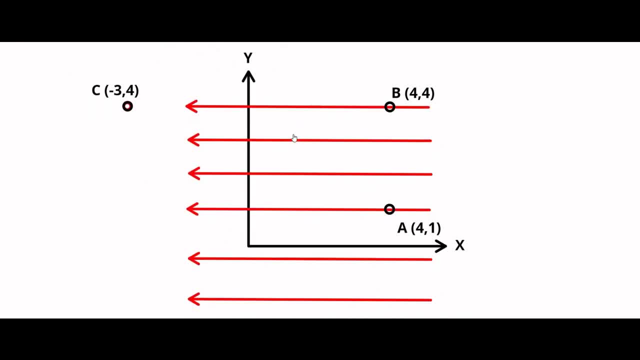 delta VCA. So first let us look at the points B and A. So if you see, they are located along the same line on the electric field. They are located along the same line along the electric field. So here, this is the electric field. So here, this is the electric field. So here, this is the electric field. 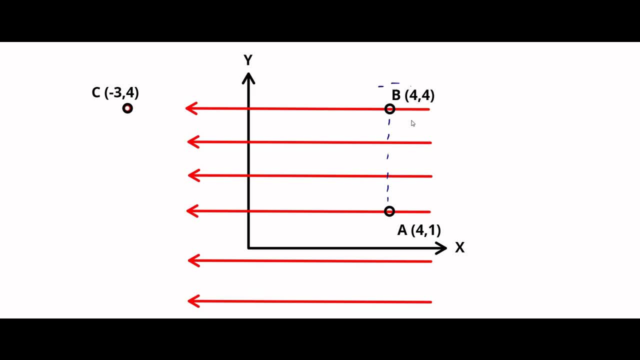 This constitutes an equipotential surface. Equipotential surface means all the points lying on the equipotential surface. they are at the same potential, which means the potential difference between the any two points on the equipotential surface that is zero. We have. 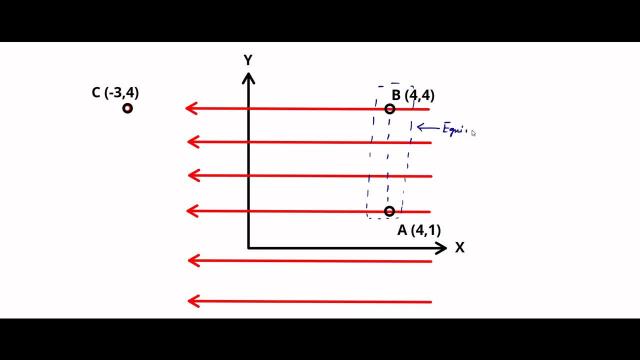 discussed about equipotential surface. You can watch the video in electricity and magnetism playlist. So the first question which is asked, to find the potential difference between points B and A. that is very simple and straightforward. No need of any calculation, anything. It is zero volt because they lie on an equipotential surface. They lie along the same line in the electric field. 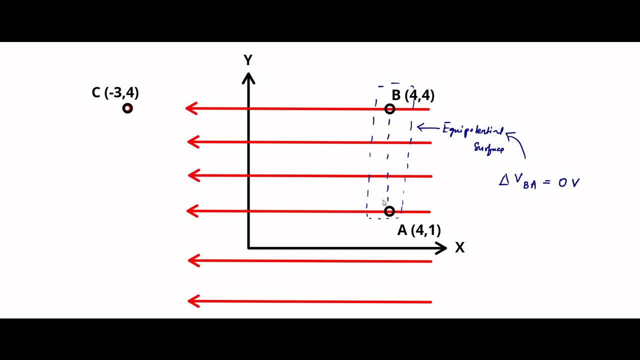 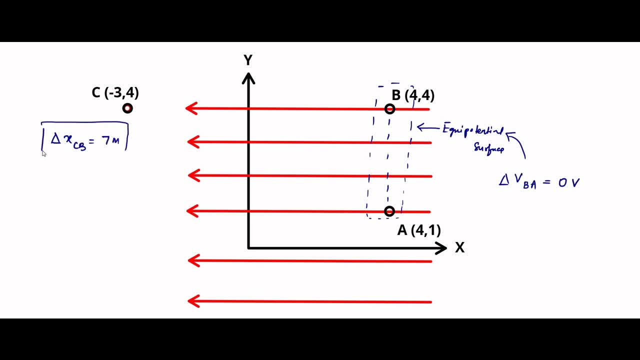 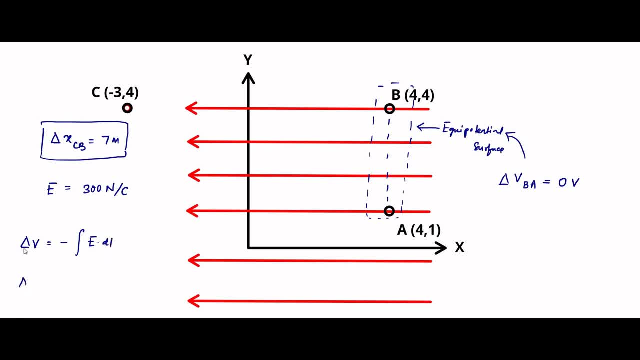 this or delta v: this is dv. this is dv, not delta v, it is dv. So delta v is equal to minus e del l, the separation, gap or distance. So here del l is del x cv, the separation. 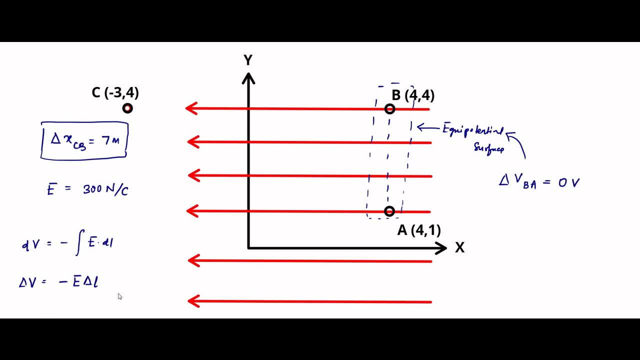 gap between points c and b. So here delta v cb, that is equal to minus e. delta x cb, the separation gap, So, which is equal to minus 300 into 7, that is equal to minus 7.. So here delta v cb is equal to 2100 volt minus 2100 volt. This is the potential difference. 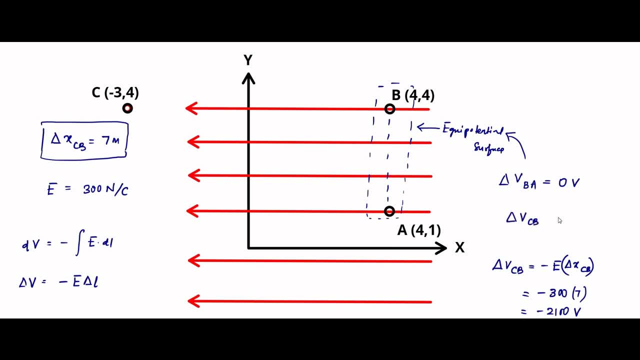 between points c and b minus 2100 volt. This is ba and this is cb. Then it is asked how to find the potential difference between points c and a. So here another interesting thing. Now here we see that point c and b: they lie. 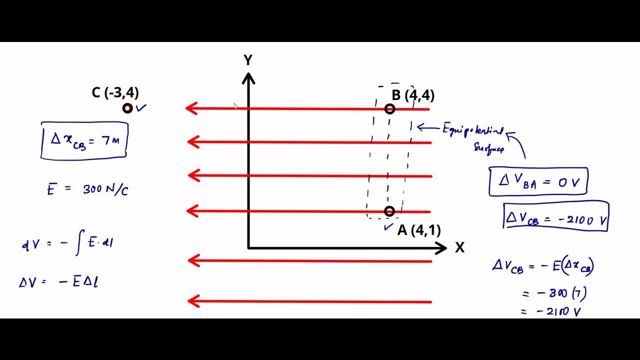 along the same line but along the electric field line direction. but here points b and a they are located along the same line but in the perpendicular direction. So here vb and Va they are equal because they lie on the equipotential surface, So as potential. 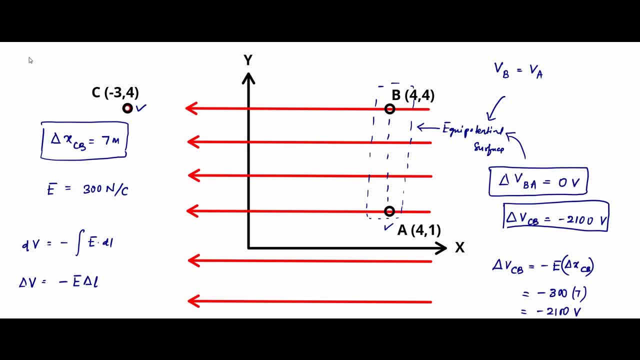 at points B and A are equal. so delta Vcb is equal to delta Vca because potential of points A and B they are the same. So delta Vcb is the same as delta Vca, which is equal to minus 2100 volt. This is the thing. So here, why points A and B? they are the same potential. 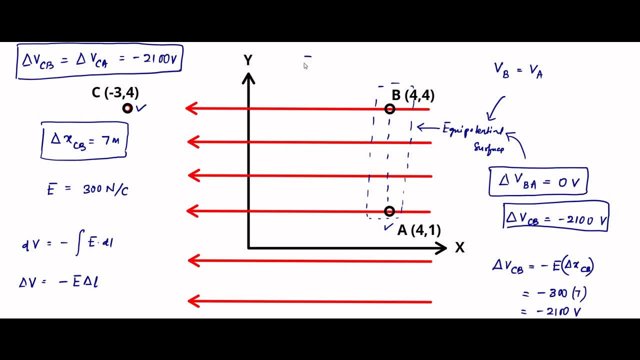 because we know E is equal to minus dv by dx. So here, as they are along the same potential, dx becomes 0. There is no change of electric field. There is no change of electric field. So they are along the same line, in the perpendicular direction. So they are at the same potential There. 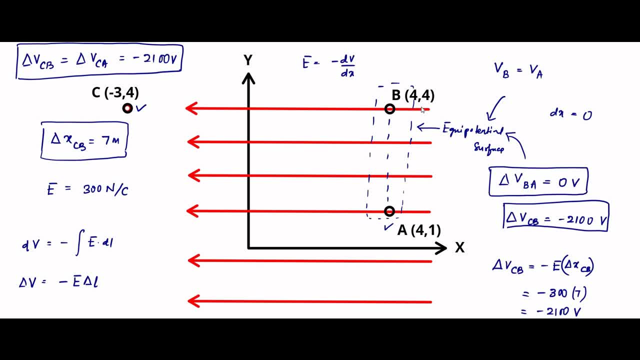 is no change in potential here. a third point is the next point. a third point is that which leads to inspirations and the other. there is a separation gap. Now, the put step on this was that delta x is equal to so and delta x is equal to minus 0. the circle will be d x, equal to plus sigma king. which is equal to 1, which gives us k, and if I divide by difficult camera and need to solve the equation between Vcb and volta. So part 2 is that is scare apply about a ratio of delta l by delta x minus 15, minus k. I would like you to understand. there is 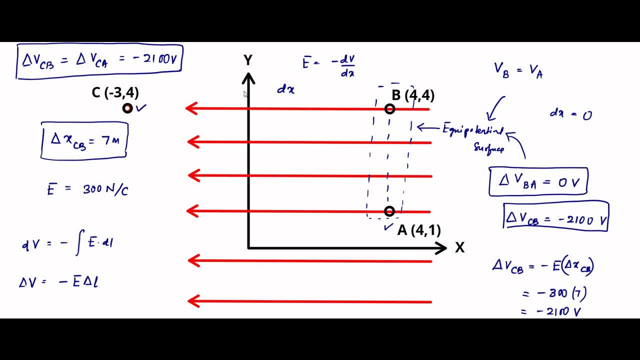 a same thing here. Here a space and platform is per another space, al k, then my equation is of k, which will be zero. So I make my equation to lambda l by delta l, delta x. this is the minimum acontecer of working as equal to zero. We will have here delta. 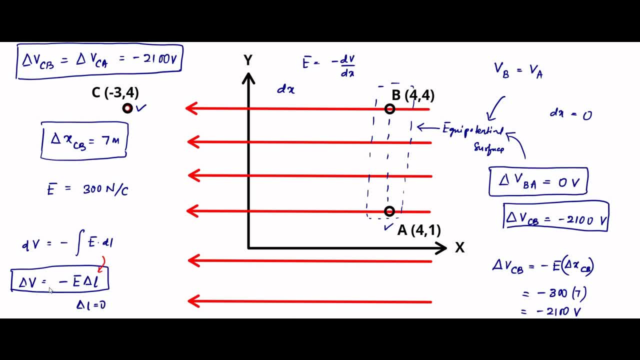 l minus s and along thiscedire ال blood. As i am using delta zdca as an advantage, the separation gap is equal to 0. in that case, any value of electric field multiplied with 0, it will be 0, which is equal to the change in potential difference. the change in potential. 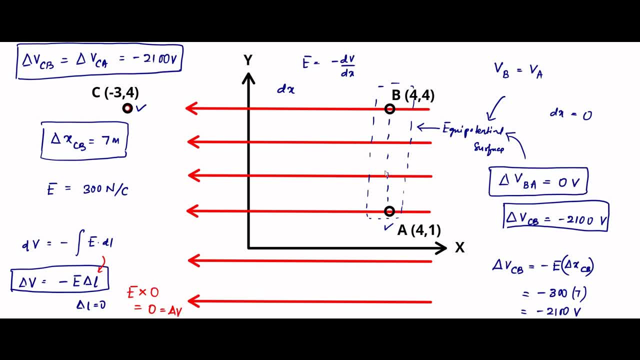 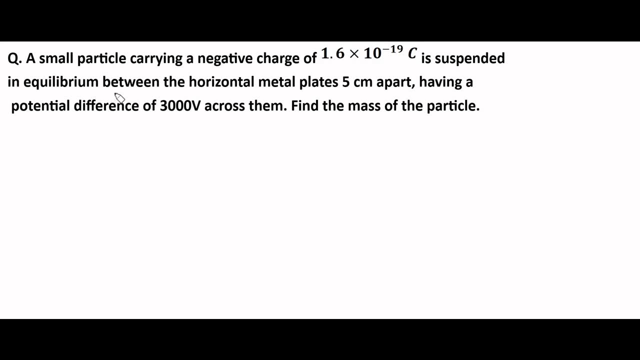 So when they are along the same line in this direction, there is no change in potential difference. they are at the same potential. So here is another question on electric potential. it is given that a small particle carrying a negative charge of 1.6 into 10 to the power 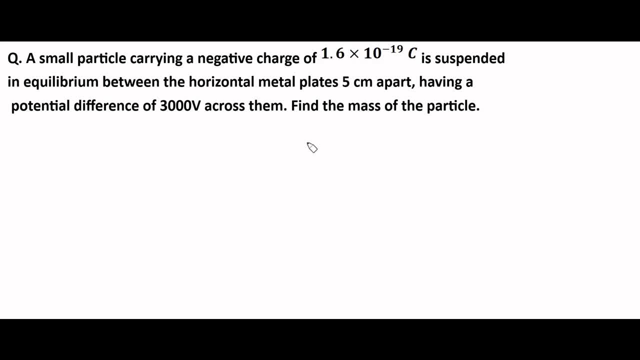 minus 19 coulomb is suspended in equilibrium between the horizontal metal plates, 5 centimeter apart, having a potential difference of 3000 volt across them. okay, Find the mass of the particle. okay, this is given. So here we have two metal plates. 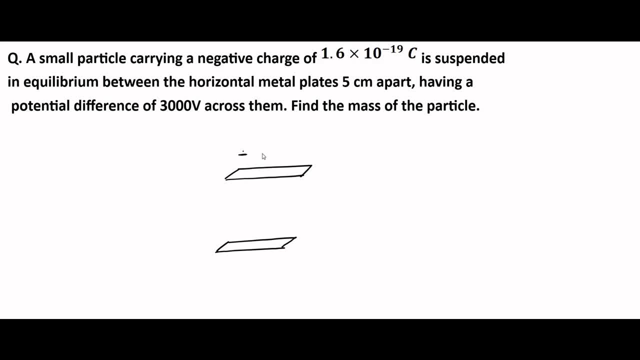 where let us say: this is the positively charged metal plate and this is the negatively charged metal plate. So here we have two metal plates where let us say: this is the positively charged metal plate and this is the negatively charged metal plate. So the electric field. 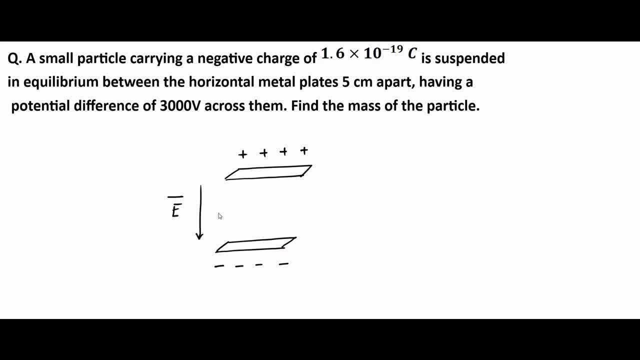 it will be in this direction. okay, Here we have a charge, negative charge 1.6 into 10 to the power minus 19 coulomb, that is, the charge on the particle mass is. we have to calculate, we have to find, So here, the separation distance. 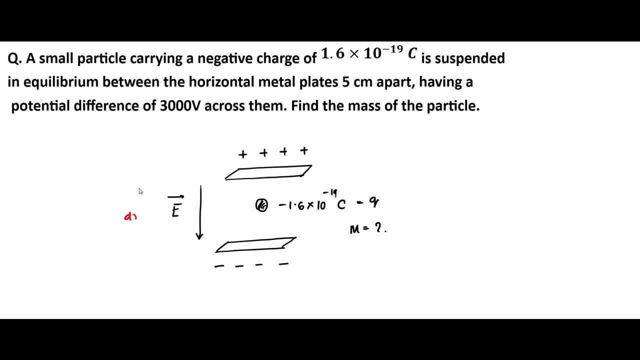 okay, let us say the separation distance between these two plates, that is equal to 5 centimeter, okay, which is equal to 5 into 10, to the power minus 2 meter, and the potential difference between them: dv. that is equal to 3000 volt. So we know electric field, that is equal to negative potential. 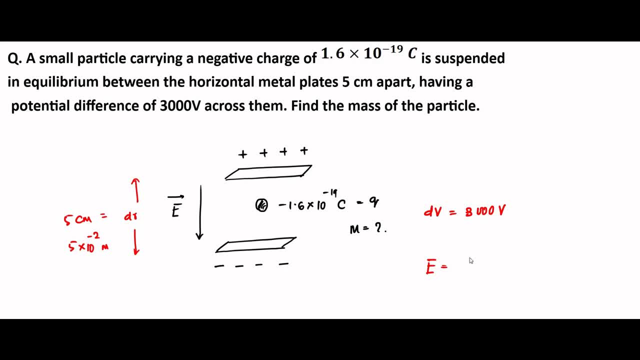 gradient. So here we are concerned only with the magnitude of the electric field. that will be equal to dv by dr. Actually it is negative potential gradient. but considering only the magnitude, that is equal to dv by dr, that is equal to 3000 by 5 into 10, to the power minus 2. 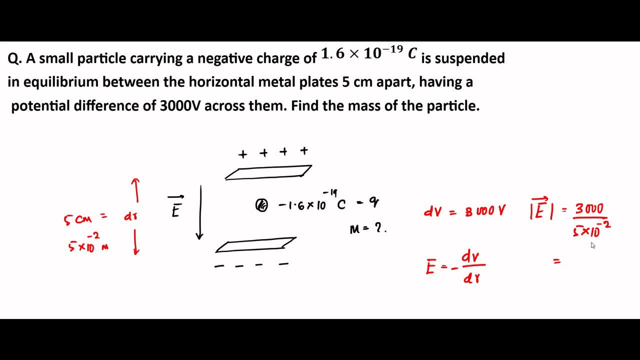 meter. So it is coming 6 into 10 to the power, 4 volt per meter. So this is the separation distance of the electric field that is equal to 5 into 10 to the power, 4 volt per meter. So this is the separation. 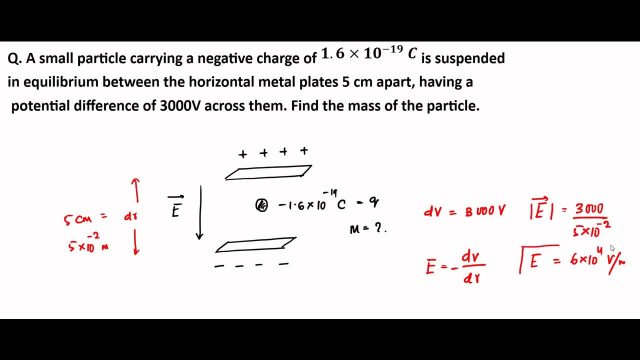 distance of the electric field that is equal to 3 into 10 to the power, 4 volt per meter. Yes, 6 into 10 to the power: 4.. Now this is the electric field magnitude. Now we know that whenever such a situation is there, it is said that it is in equilibrium. 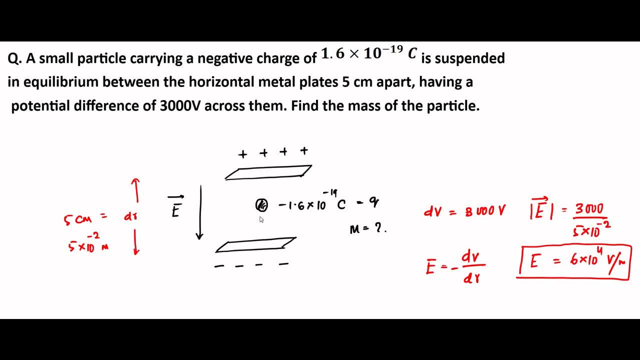 Equilibrium means it is not moving either upwards or downwards. It means two forces are acting on the tail: because of its mass and acceleration due to gravity, a downward gravity force, mg, and as it is a negative charge, it will experience a force of repulsion from the negatively charged plate at the bottom. So an upward repulsive electric. 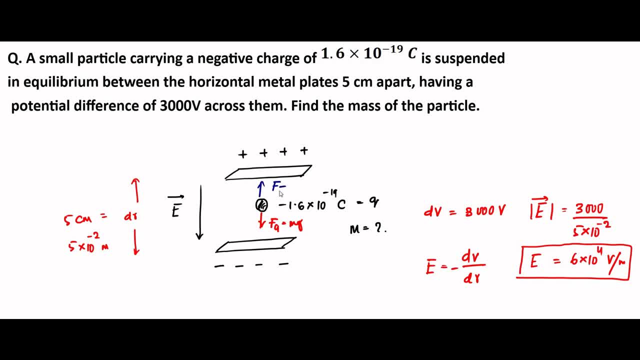 repulsive, electrostatic force of repulsion. So, since it is in equilibrium, the electrostatic force that is equal to the force of gravity, The electrostatic force we know that is equal to q e. ok, q e and this is equal to mg. So q e is equal to mg at equilibrium. 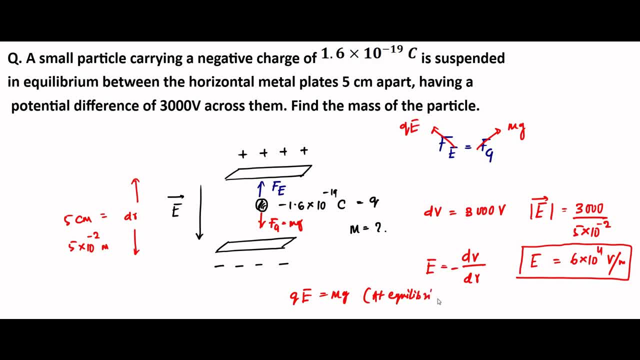 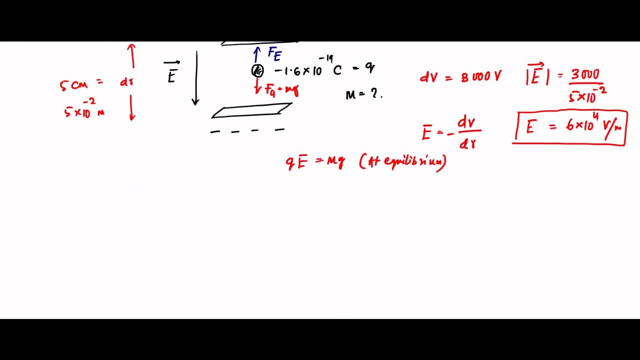 ok at equilibrium. that implies the mass is equal to q e by mg. sorry, q e by g, sorry, q e by g. this one will not be there. q e by g, only q e by g, which is equal to 1.6 into 10, to the power minus 19 coulomb. consider: